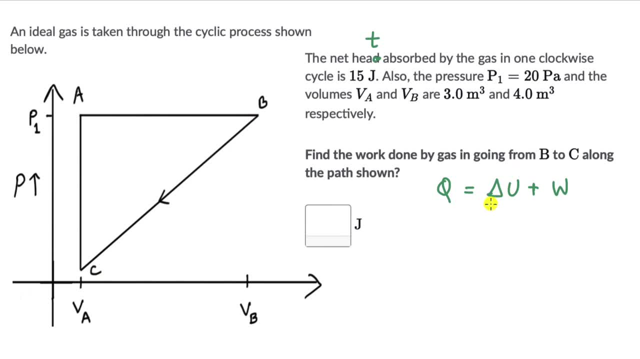 here, because this is a cyclic process, we can say that delta U will be zero because it starts- let's say it starts from C. It starts from this point which has some pressure and volume. That means this state will have a temperature because it has a fixed pressure and it has a fixed volume. And 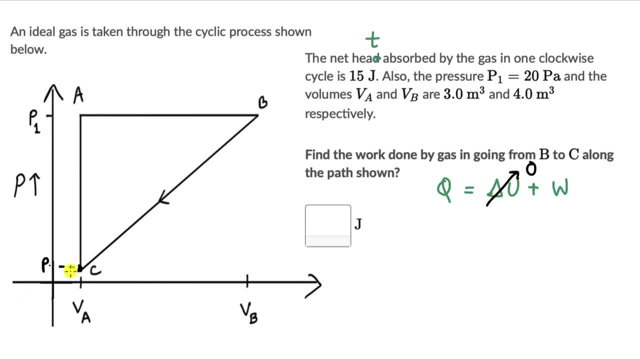 now the system comes back to this state C after going through the cycle. So it comes back to the initial state, which means the same temperature that it began with. When the temperature doesn't change in your entire journey, then it means there is no change in internal energy. So we can say that. 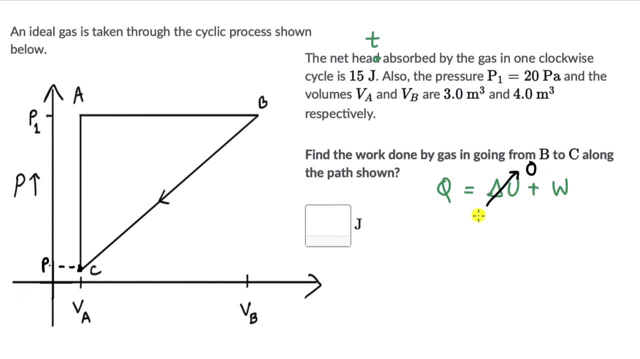 delta U really is zero for any cyclic process. So that means that all the heat that was absorbed by the gas, that is equal to the work done. So Q net, we can write. Q net is really equal to W net And this is equal to 15 joules, which is given in the question. that is, this is 15 joules. Now we need to. 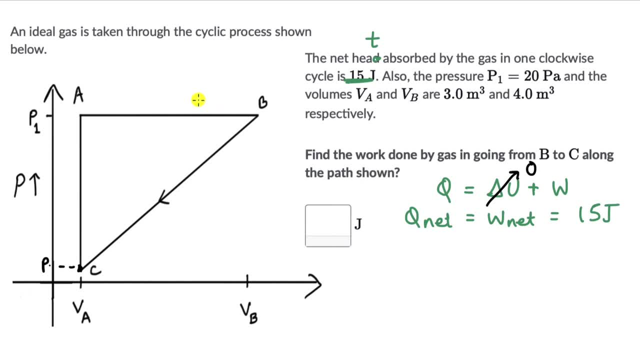 figure out the work done for one path. So let's divide the cycle into three parts: AC, AB and BC. So work the network done. this is really equal to work done in the process C, A plus work done in the process AB, plus work done in the 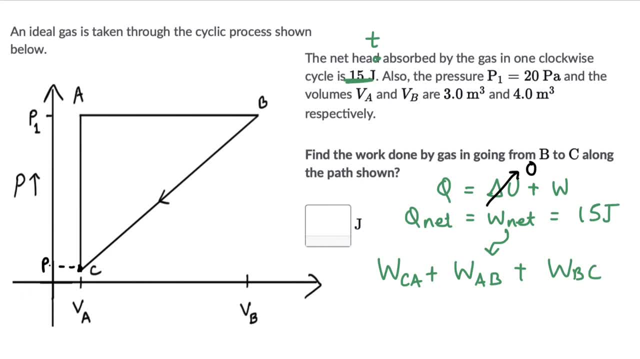 process BC. Now we need to figure out the work done in the process BC. So this is the, this is the question mark: work done in the process C A. Let's look at C A. So here there is no change in volume and work done is given by P, delta, V. 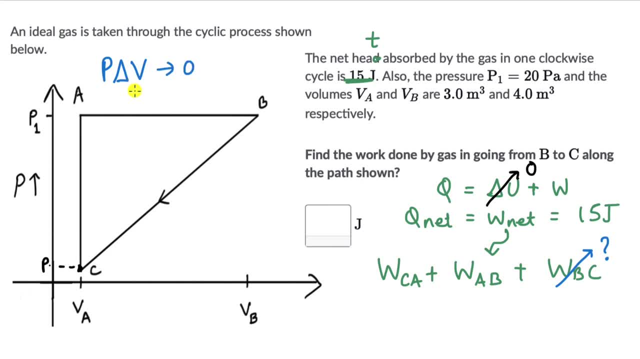 So this is only true when A bend is zero because there is no change in volume. Well then, will also be zero. This is only true when delta V is zero. Alright, so work done in the process, CA, zero, work done in AB. now, this is AB. it has one pressure and volume is changing. So let's use P delta V for 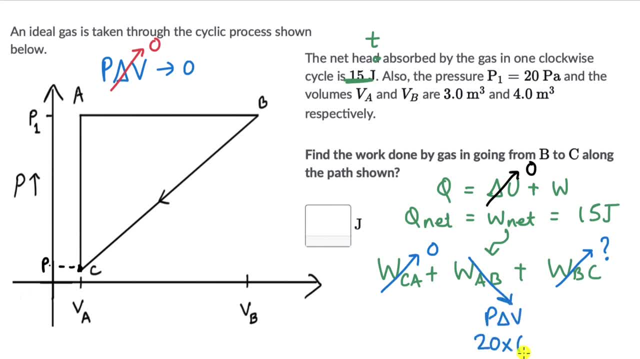 this one. This is P, delta V. P over here is 20 pascals and delta V will be 4 minus three VB minus VA. So 4-3 is 1. 20 joules. so net work turn that is 15, 15. this is equal to work turn in the process a, b which came.